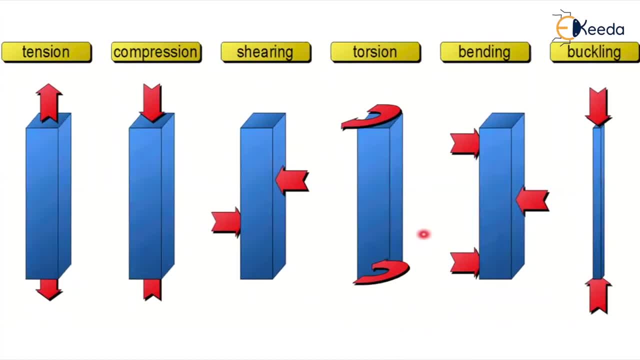 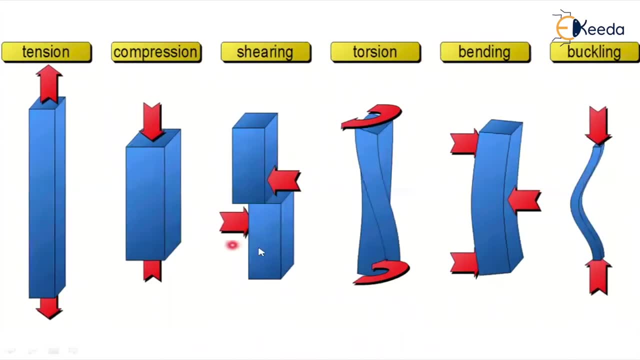 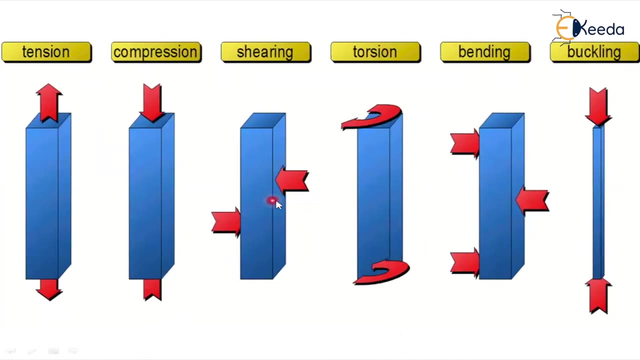 All these things we are going to discuss in this session. So let me introduce first of all strain hardening. What do you mean by strain hardening? It is also work hardening or cold working process, making a metal harder and stronger through plastic deformation. 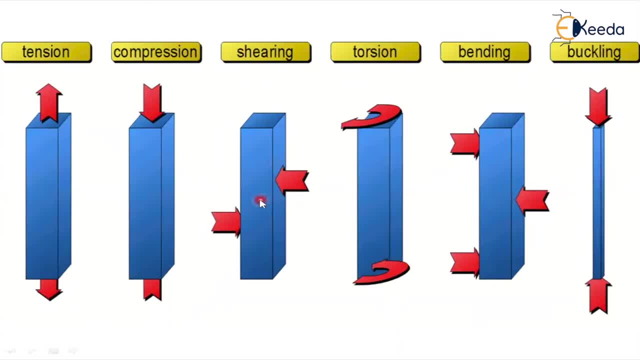 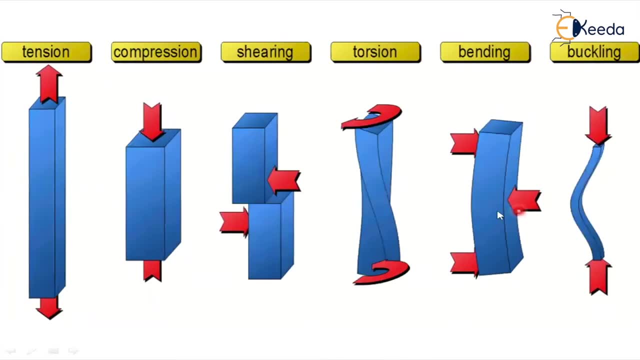 Means when a metal is plastically deformed. like this You can observe The various plastic deformation process. All these are plastic deformation process. only When a metal is plastically deformed, dislocations move and additional dislocations are generated. So that means when the dislocation moves from one place to another place if the load is applied. 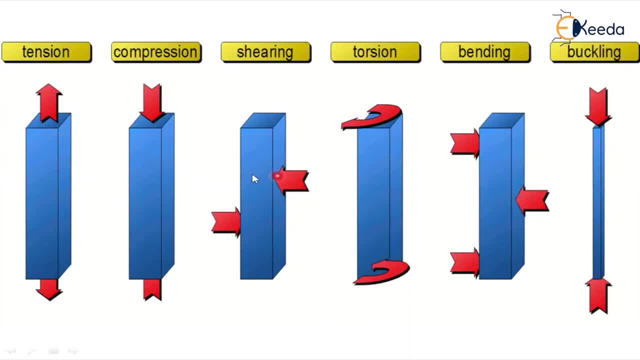 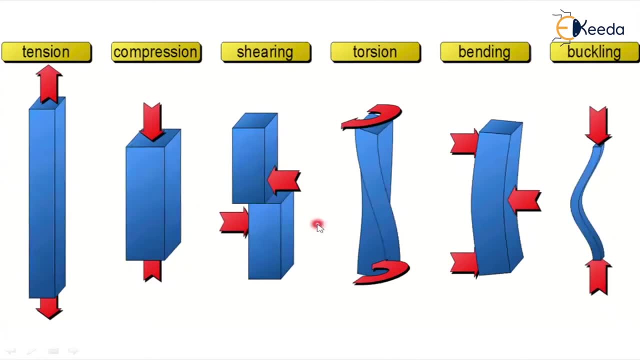 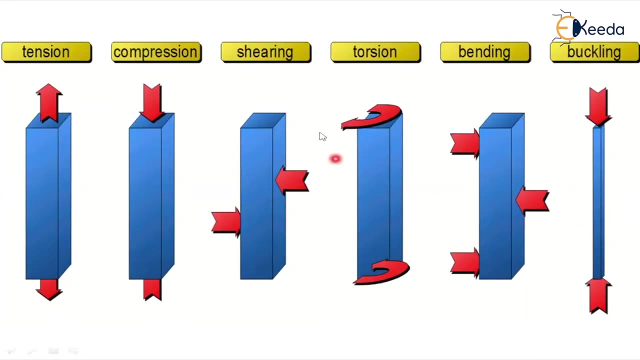 Automatically what happens. New dislocations may be formed. Our analysis is concentrating how there is dislocation, How these dislocations are going to be utilized, Or how these dislocations are helpful to a metal in becoming stronger. So that is our analysis. 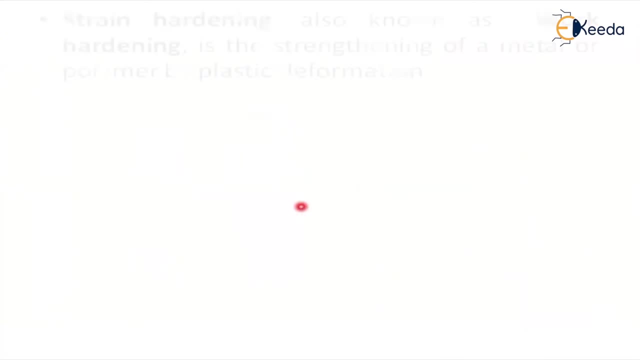 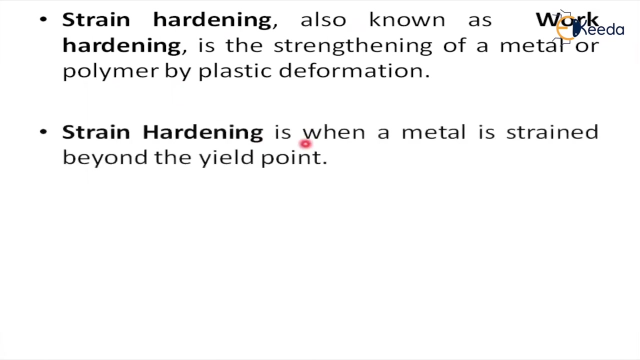 Next, Here you can observe the salient features. first, What do you mean by strain hardening? So I already said it is also known as work hardening. It is the strengthening of a metal or polymer, Or polymer by plastic deformation. It is when a metal is strained beyond the yield point. 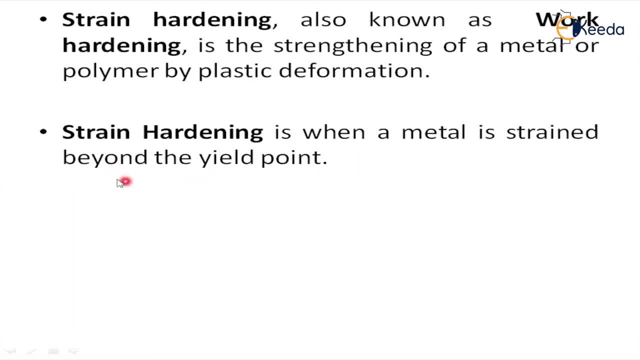 This point is important. That means when the metal is strained beyond the yield point, This strain hardening stage is going to be started After the yield point only If you increase the stress. So whatever the stress is required, The minimum stress is required. 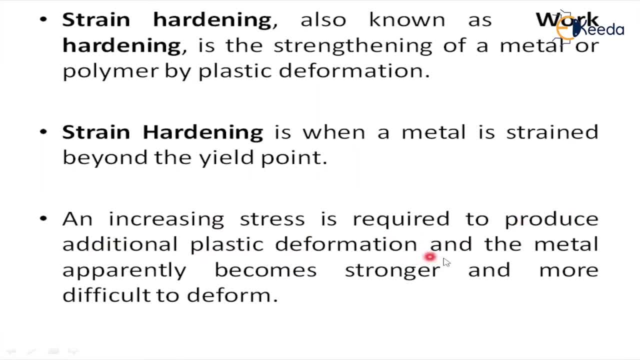 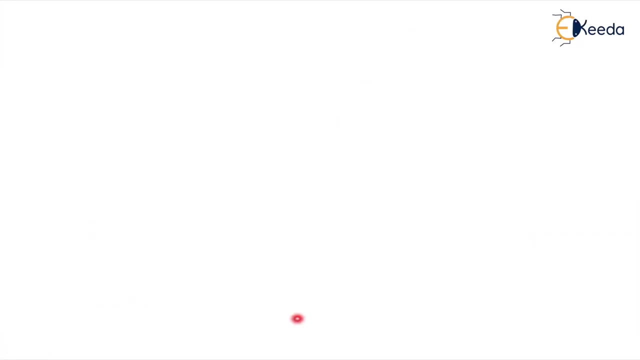 Which produces additional plastic deformation And the metal apparently becomes stronger and more difficult to deform. So that means if the stress is continuously increasing, Then the material becomes stronger and stronger And it is very difficult to deform. Observe the image here. This is the dislocation area. 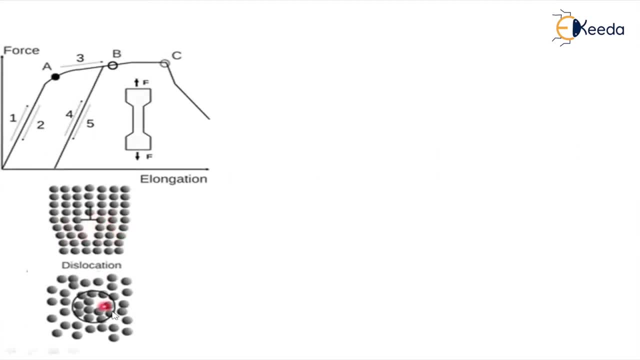 This is the edge dislocation, And here you can observe A circle In which all the atoms are disturbed At one region. When void space is generated, All the atoms wants to come And wants to occupy that region Automatically when the other atoms wants to come. 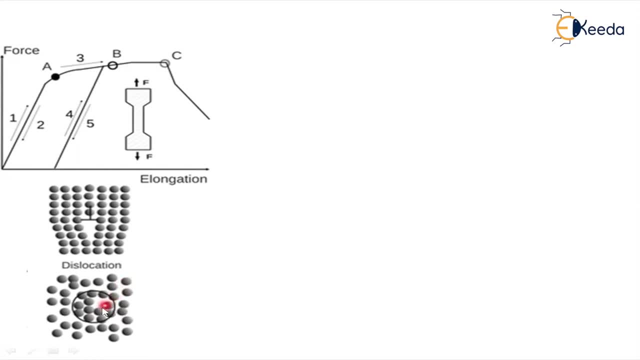 And wants to occupy in this region, Then here some disturbance. Some new dislocations may be generated. So this is the dislocation area, This is the edge dislocation And here you can observe If new dislocation is generated Again, here another disturbance is observed. 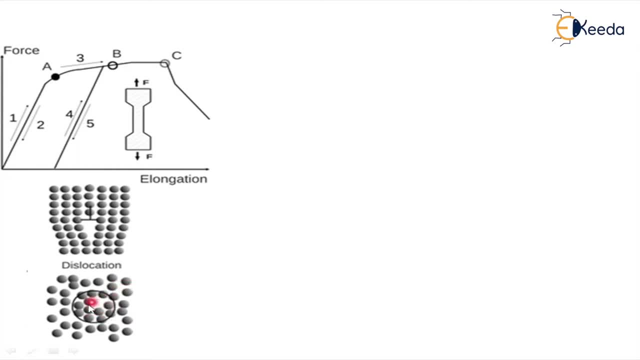 So that means one dislocation May cause So many number of dislocations. This particular point Is very, very important In understanding strain hardening Up to That is, Stress is directly proportional to strain Up to some point. So that is up to yield point. 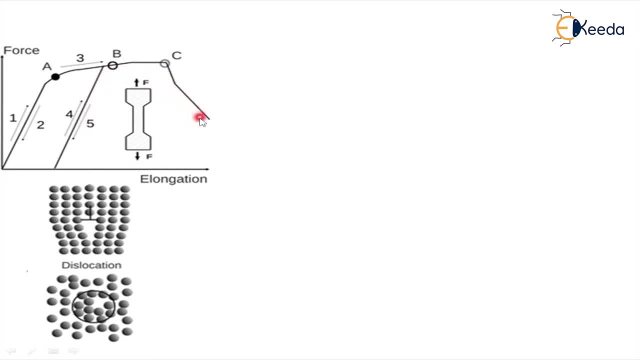 After that the plastic region Is going to be Formed. So we have to do some analysis In the plastic region only, Not in the elastic region, How the strengthening occurs here. So please observe the sentence: here The strengthening occurs. 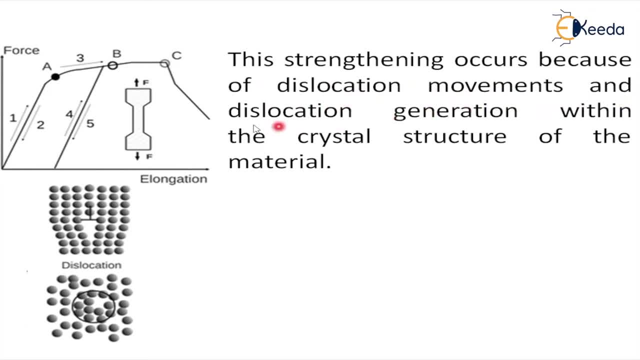 Because of dislocation movements And dislocation generation. So that means These two are important: Dislocation movements And dislocation generation Within the crystal structure of the material. And one more point Here: Whatever the dislocations are generated, 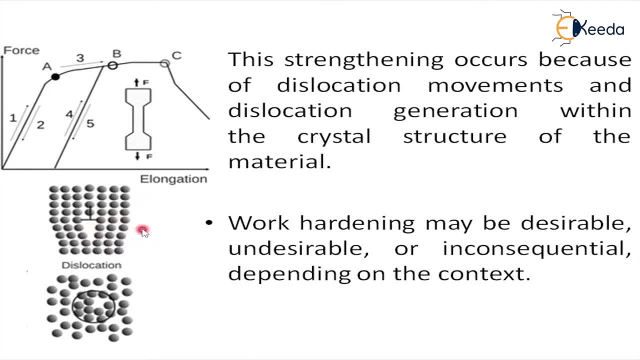 Sometimes this is useful. Sometimes these dislocations May not be useful for the material. Useful means: If the dislocation helps To increase the strength of the material, That is useful. If the dislocation is not helping In increasing the strength of the material, 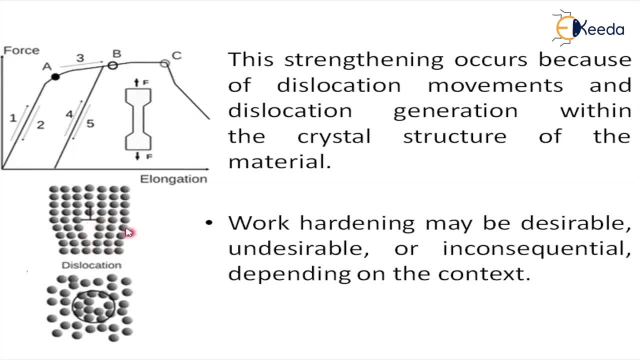 In another words, If it causes In reducing the strength, Then it may not be useful, It may not be desirable, Undesirable Or inconsequential, Depending on the contest. So that means completely depends on the usage, The final usage. 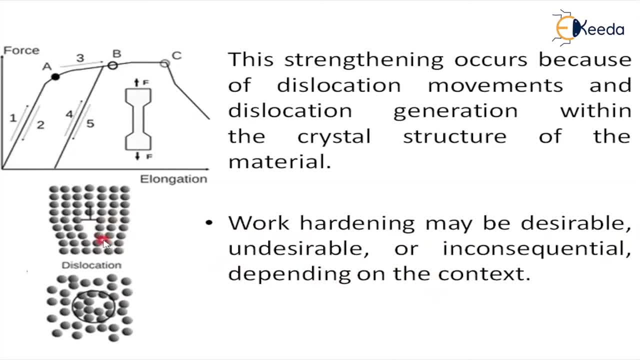 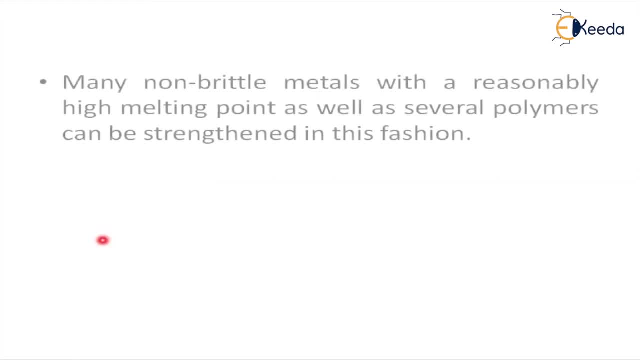 We can say that This type of straight hardening May or may not be Useful. Observe some more salient features. Many non brittle metals With a reasonably high melting point, As well as Other polymers, Can be strengthened. 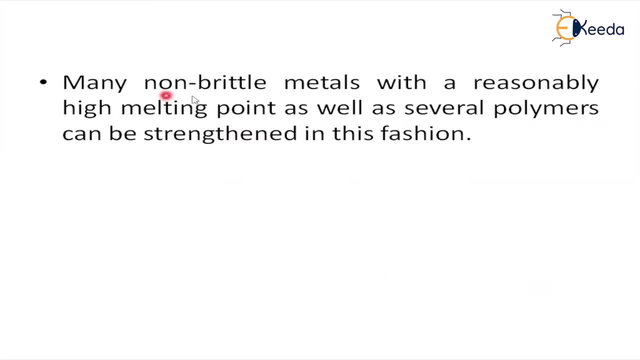 In this fashion. So that means This is a very, very simple process. First, generate dislocations Automatically. one dislocation, Increase another dislocation. Then, with a reasonably high melting point, Automatically The many materials Can increase its strength. And the main problem is: 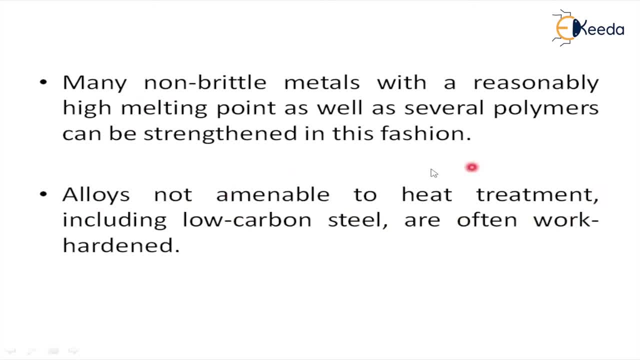 Some materials may not Increase its strength To heat treatment, So for those materials This particular straight hardening Is the best process. So you can see that Alloys not amenable to heat treatment, Including low carbon steel, Are often work hardened. 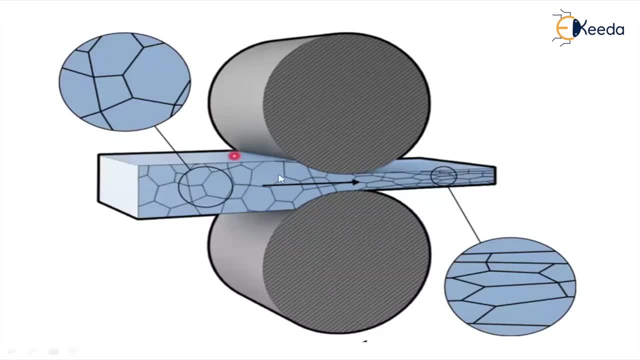 You can observe the image here How the straight hardening Affects the material Before rolling process And after rolling process. These are the grains You are observing on the surface. You can observe. the Grain surface Is the microstructure of the grain surface. 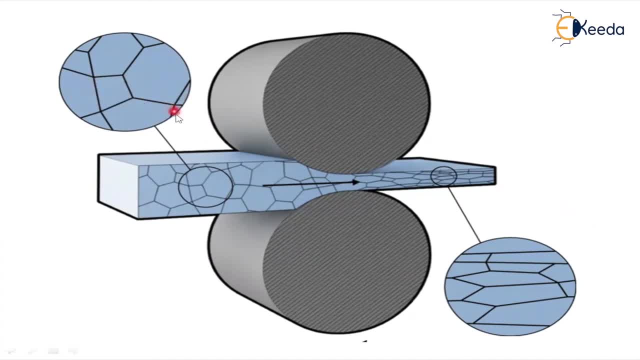 All are All. grains are widened, But after rolling process The grain size, The grain surface area is decreased. What happens If the grain surface area is decreased? Suppose if the dislocation Is existed here, Automatically The movement is restricted. 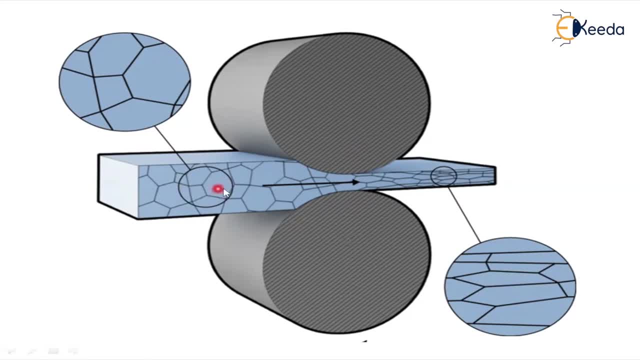 Here the dislocation movement Is not restricted. here The widened space Gives the free movement Of the dislocation Suppose. if the dislocation movement is restricted, Automatically the material becomes stronger. Suppose: see: All the dislocation movements May be restricted. 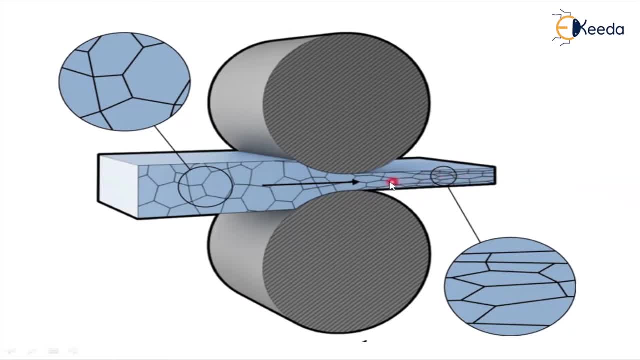 Because of the reduced Grain size area. So this is the main Mechanism In generating The strength of the material. So this is the main point Of strain hardening. So that means we are Seeing that how does Work? hardening increases. 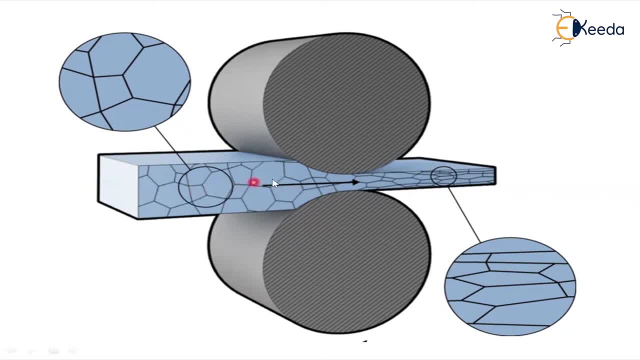 Its strength. It deliberately, by hammering Or rolling or drawing Or any other physical process. Automatically it increases Its strength. In another words, this rolling process Induces strength in the Material, Although the first few deformation Imposed on a metal by such treatment. 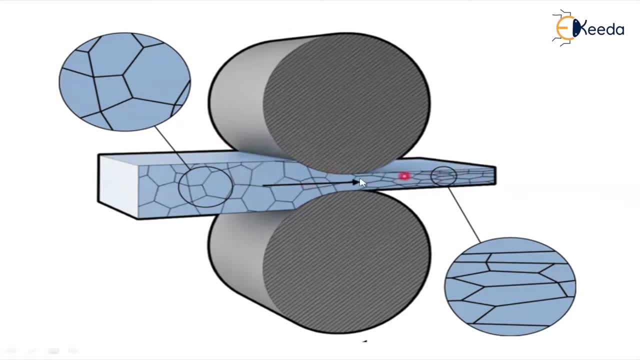 Weakens. its strength is increased By continuous deformation. So that means At first time The strength may not be increased By passing several times. It may be rolling Or drawing or any other physical process. By doing several process, The strength of the material 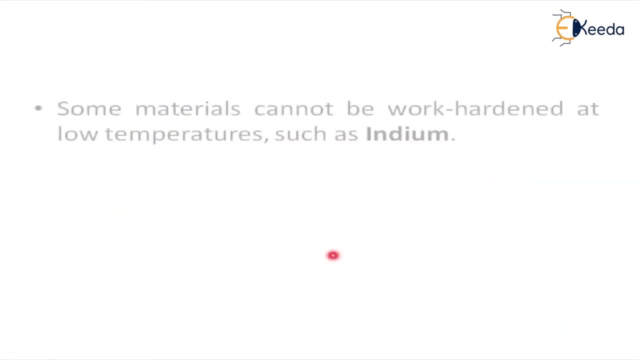 May be increases. You can See the important point here. Some materials cannot be work hardened At low temperatures, Such as indium Indium is the example. At low temperatures It cannot be work hardened, However, Thus can only be strengthened. 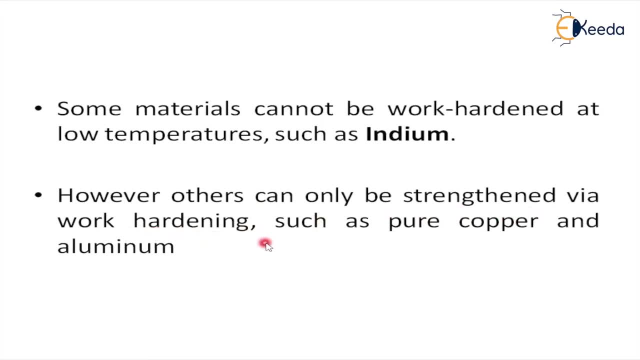 By a work hardening. So that means completely Depends on the work hardening only, Such as a pure copper And aluminium. So that means only The work hardening process, The copper and aluminium, can be strengthened. So that means 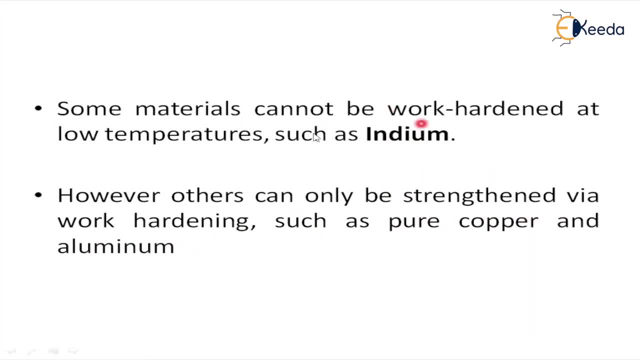 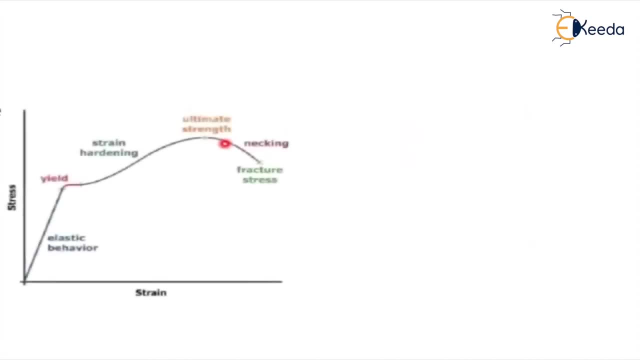 This is the best example- And indium is the best example At low temperature, Which cannot be work hardened. Observe the graph here, The various regions You are observing, The typical regions: Stress versus strain Up to some point. 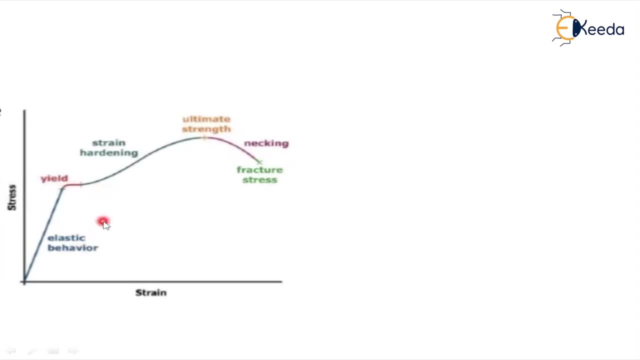 Elastic behavior And then, After yield pointing is completed, Then A curve rises like this. All these are typical regions That can be observed in stress strain curve. The first one is elastic region, The next one Is yielding, The next one 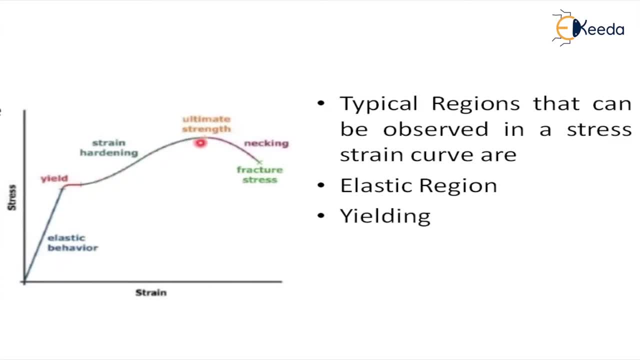 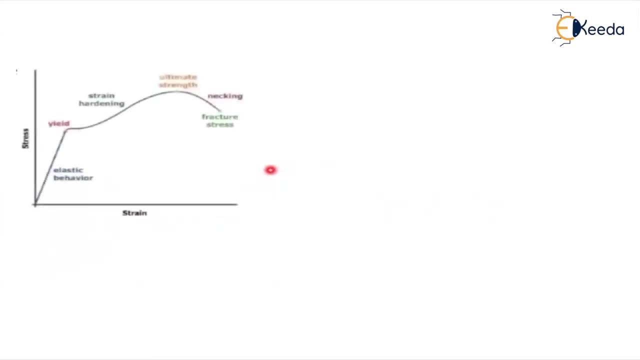 Is strain hardening Like this: The next one is necking, The last one is necking And after that, Failure. These are the various regions Observed In this graph: Stress versus strain graph. The main point is: 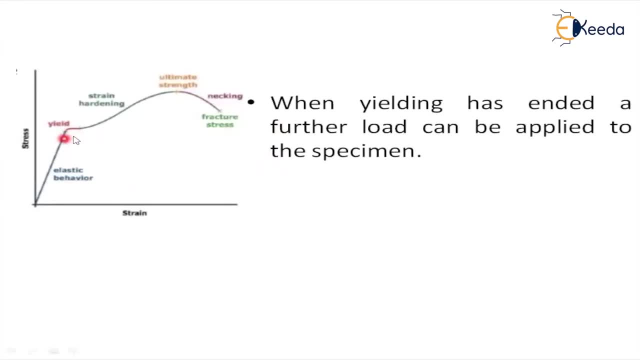 When yielding is ended. Here, When the yielding is ended, A further load Can be applied by the specimen. So here the yielding is ended. here, When the yielding is ended, Further load Is applied on the specimen, Resulting in a cure. 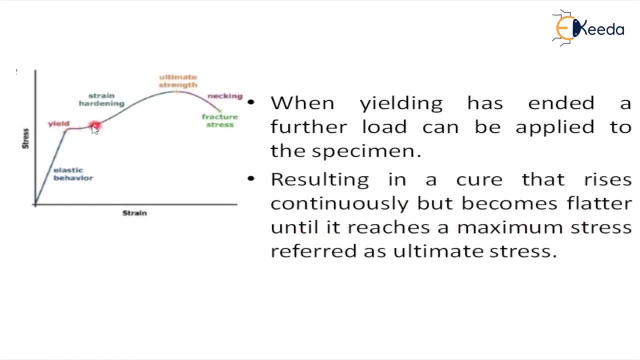 Continuously But becomes flatter Until it reaches The ultimate stress, Or strength here, Until it reaches ultimate strength. So this region Is called as a plastic region. In another words, It is the region of strain hardening Region. 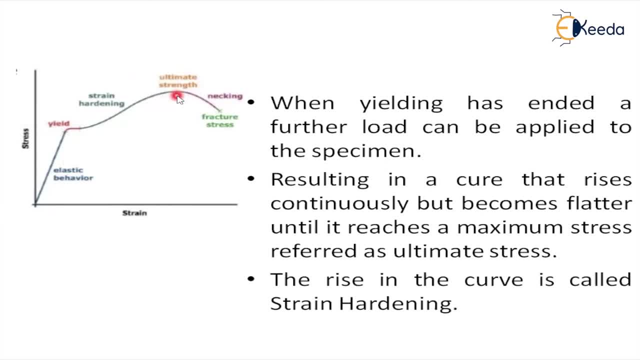 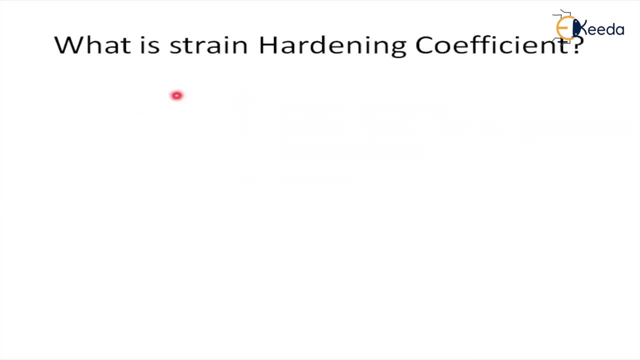 So that's why this rise In the curve Is called strain hardening Here. So many effects are there. So that means What is the strain hardening quotient? So we are going to observe The strain hardening quotient Here we can say: 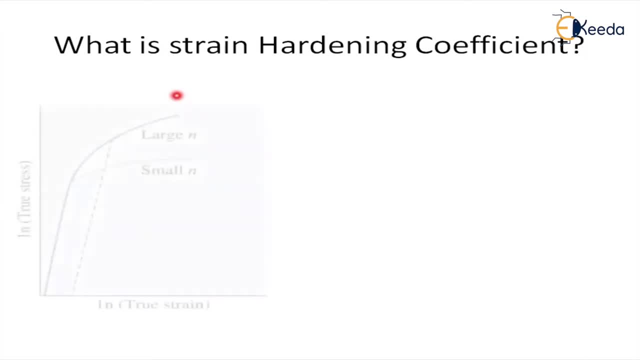 What are the advantages, What are the various advantages Of strain hardening? So that means It increases the material. The main advantage of strain hardening is It increases the material hardness By restricting The location Movement. Now, what is quotient here? 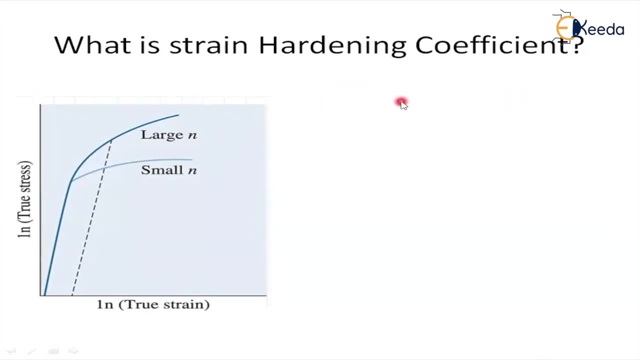 Strain hardening quotient. It is a parameter of strain hardening. How much the value, How much strength is going to be increased For a particular material. Exactly what do you mean by Strain hardening quotient here? It is a measure of how much metal. 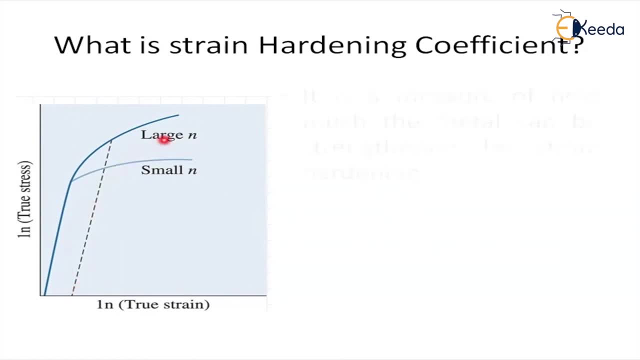 Can be strengthened By strain hardening. So that means it is a measure, The value which shows. Maybe suppose If the curve is like this, The material can be Hardened or strengthened Up to this level only. So that means 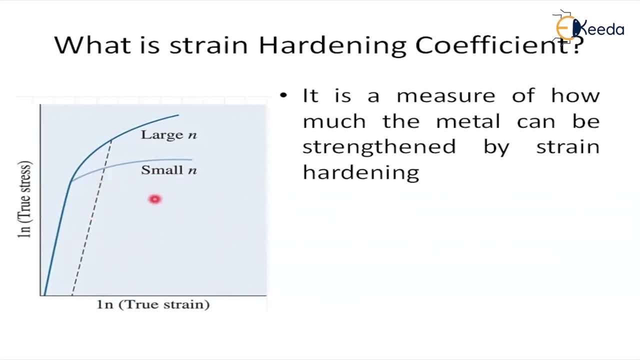 If the area decreases, If the area is low, Then we can say that The material cannot be hardened Beyond this value. Suppose if the area, If the grass shows. This is the large N here, The quotient This particular Material will give. 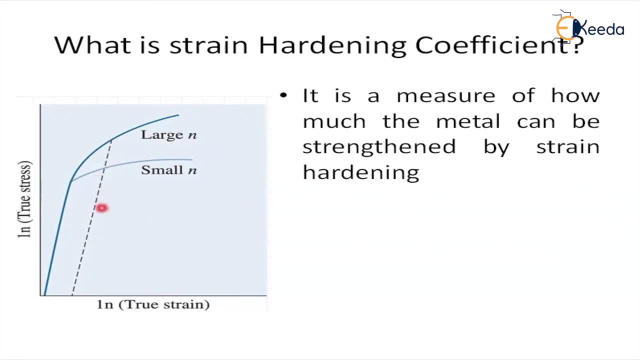 Maximum strength. The main Intention of the strain hardening Is by restricting Dislocation moment We can increase the Strength of the material. That is the main logic behind Strain hardening. Some materials may not accept The strain hardening. 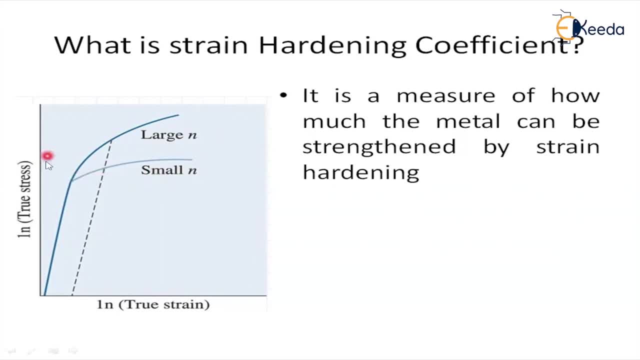 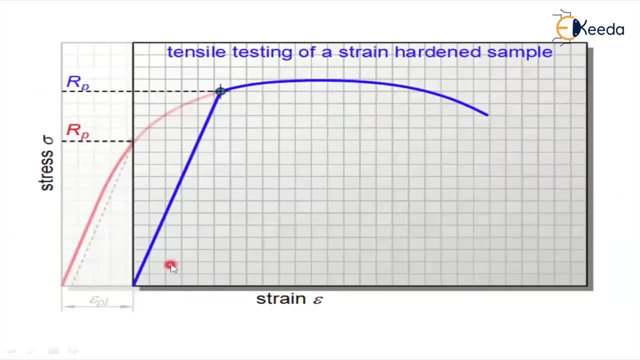 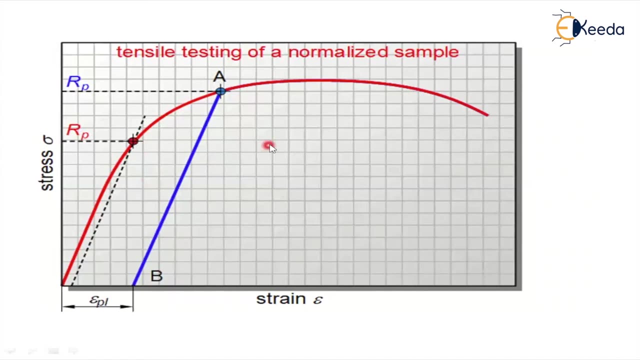 Sometimes due to this strain hardening, Sometimes the material may Not show the strength. That may be happened, But maximum material shows Its strength. You can observe in another graph Is the graph. here You can observe clearly How the tensile 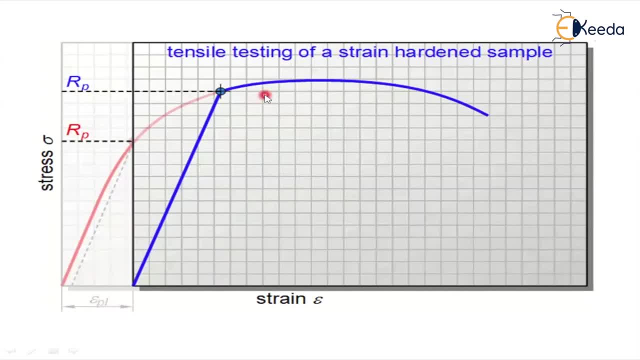 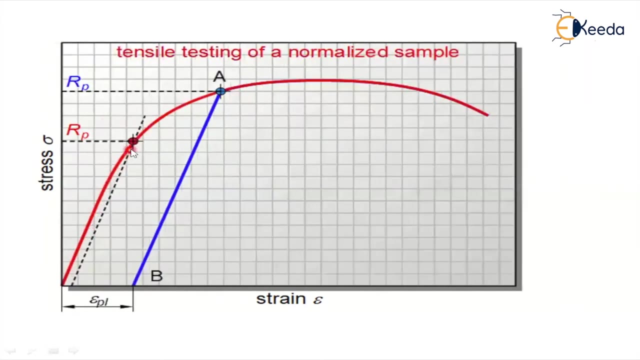 That is, in a tensile testing Of a stressed, hardened sample. So this is the This blue color. So up to this The material is strained Here. This is the general Form. The material is directly proportional. The stress is directly proportional. 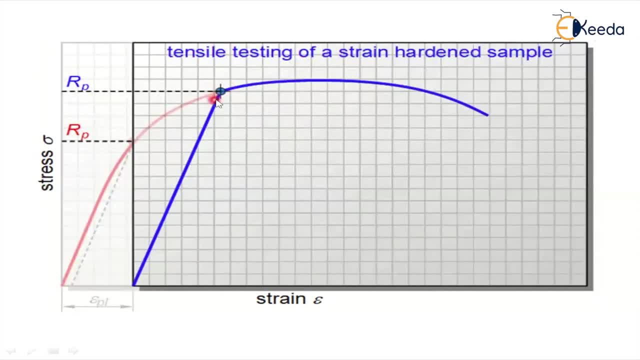 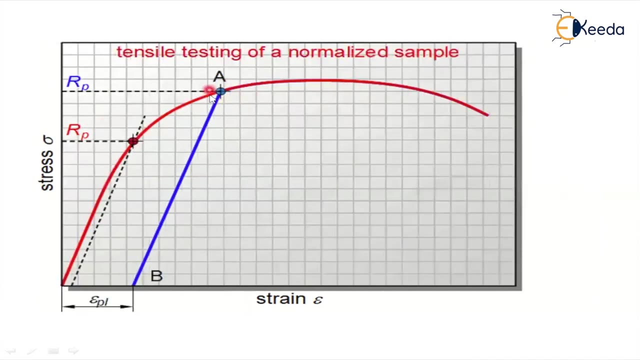 To strain up to some level. After that This is up to yielding point, Then after yielding point. So this is the end point of the yielding point. Then the plastic region starts. For any material, The plastic region starts After the yielding point. 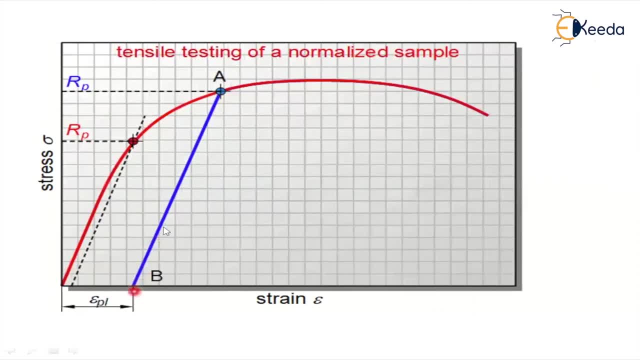 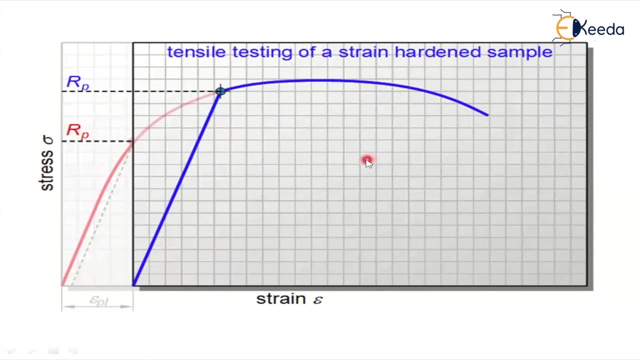 Completes. So many advantages Are there for strain hardening. Not only one Advantages here, And this is also called as Work hardening zone, Work hardening zone Or strain hardening zone. Strain hardening region or zone. 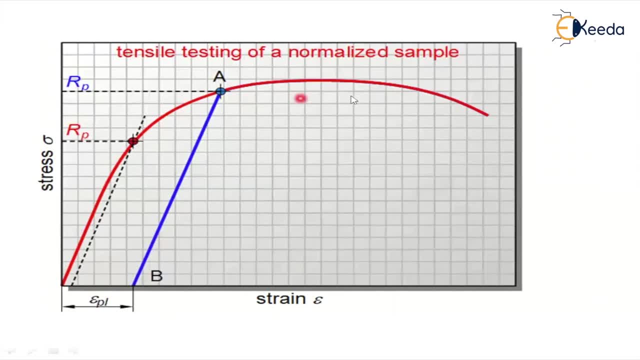 Means it is the region between yielding point To ultimate strength. That is called as Strain hardening Because this region- Cow shape- depends on the strain rate. So that means if the strain rate increases, This cow also comes. Depends on the strain. 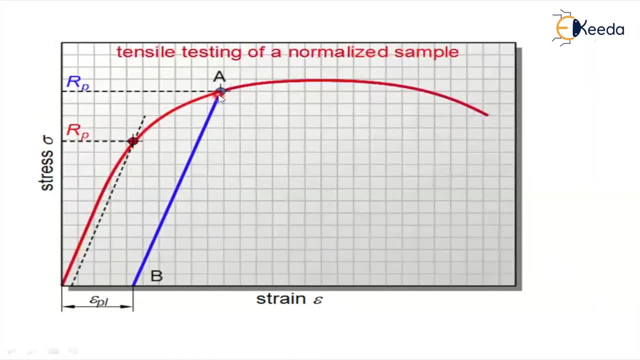 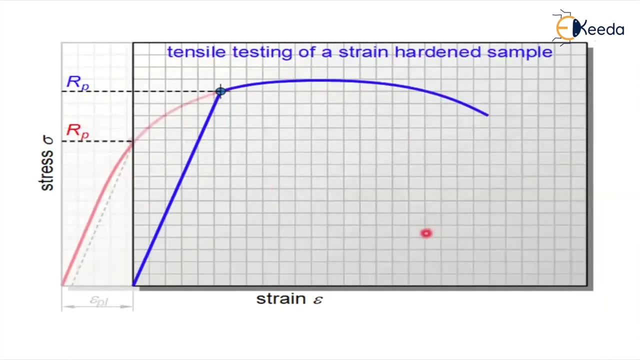 Value, And sometimes we can say that What is a hardening material? Hardening? Hardening is a metallurgical Metal working process Used to increase the hardness of a metal. So many advantages Are there. This is all about.